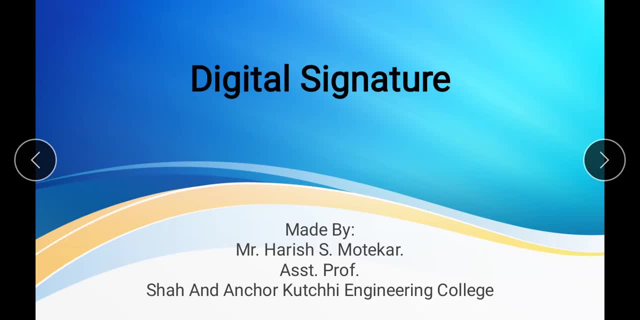 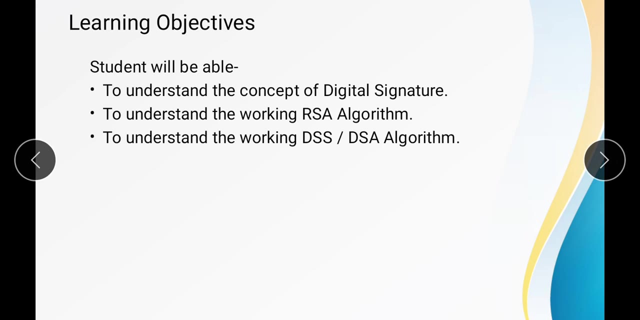 Hello students. myself, Mr Harish Salashu Motekar, I am your subject teacher for the subject Cryptography and Network Security, And our today's topic is Digital Signature. Okay, so, before starting with the topic, let us see the learning objectives, And the learning objectives are: after learning this lecture, student will be able to understand the concept of digital signature. 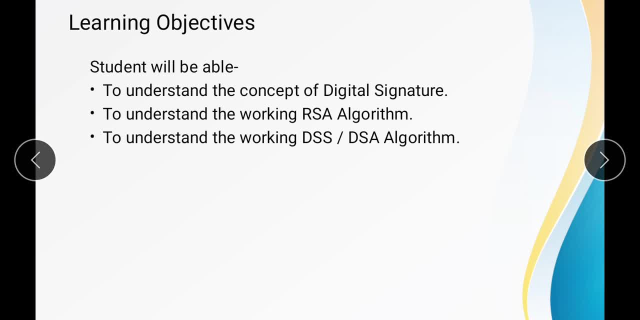 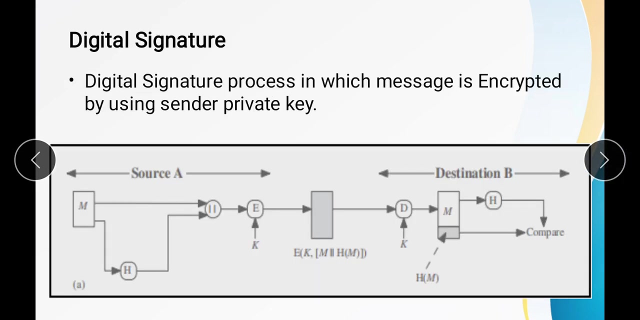 Second one is the student will be able to understand the working of R-S algorithm. And third one is the student will be able to understand the working of D-S-S or D-S-A algorithm. So these are the learning objectives of the lecture. Now let us start with the introduction to the digital signature. 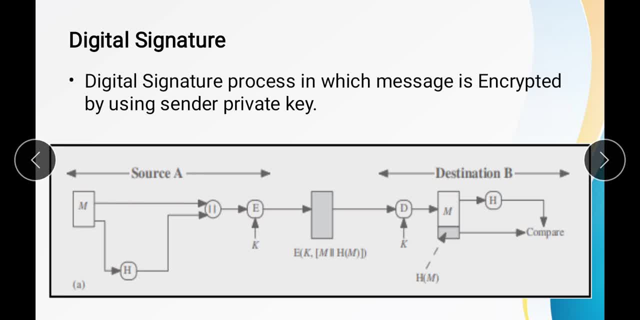 So suppose we have two users And one is sender and another one is receiver. Sender wants to send a message to the receiver and for that he uses his own private key, So that he is using the private key for the encryption. 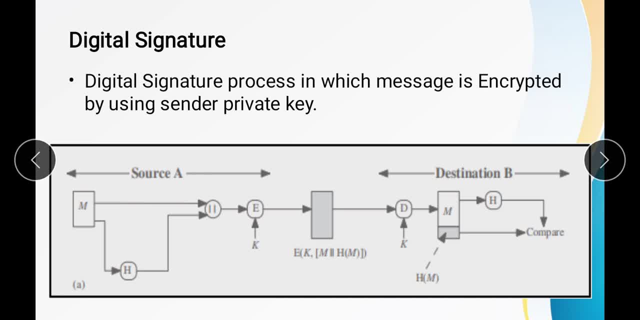 On the other hand, receiver is receiving that key, that message, and decrypting the message using the public key. So this technique where we are using private key for encryption, Private key for encryption, that known as the digital signature technique- We can understand this whole process using the diagram which is given below. 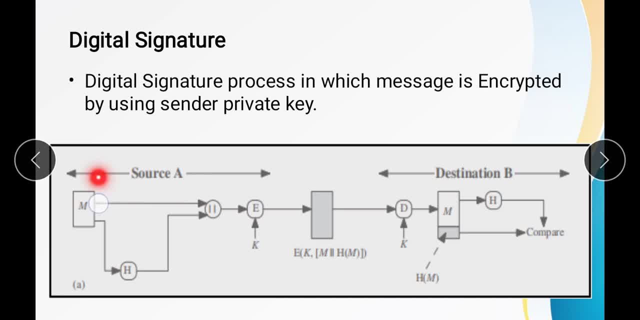 So suppose we have a source, that is sender, suppose, and destination, which is a receiver, So sender wants to send a message. That message is M, So he wants to send a message by using the digital signature technique. In that case, first he encrypts the message. 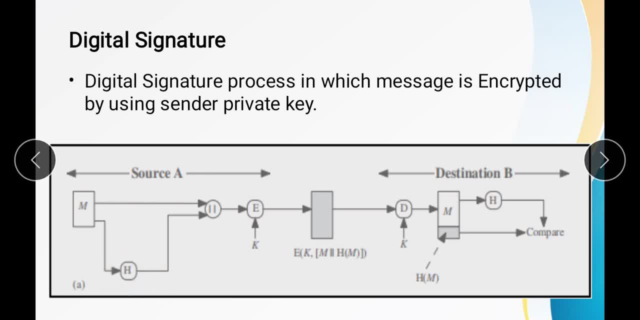 And generates a hash. That hash is then appended with the message And that part- that message- is encrypted using the key that is K. So we got a message that is encrypted with the key K. So it is a hashed message which is encrypted with the key. 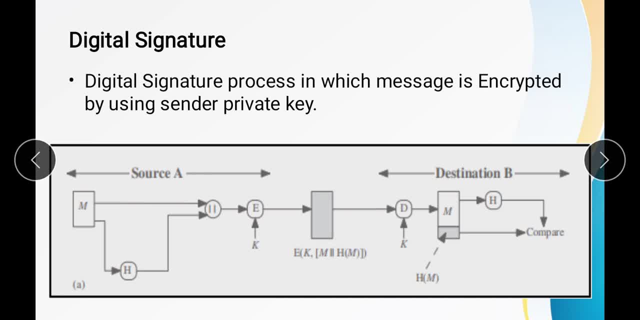 Now that message is sent to the receiver. That message is sent over the network- that is secured network, surely, And which is received by the destination or receiver, And the receiver first decrypt the message. Decrypt the message using the public key: See sender. encrypt the message using the private key. 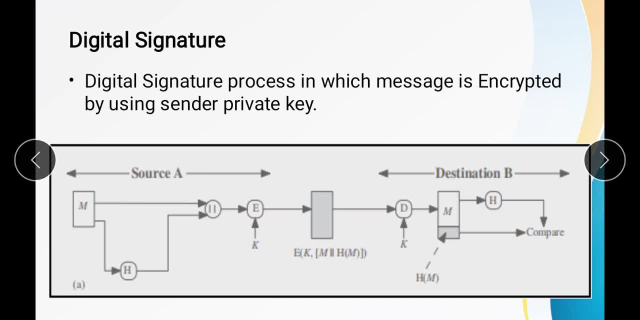 Receiver, decrypt the message using public key. And now that message, After decryption, we get the message in which the first part is M, That is the message, And second part is what Hash That we have seen earlier here. So that hash after the decryption. 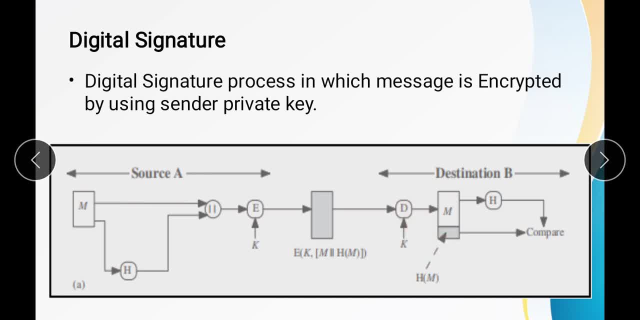 So now user will compare the hash with the existing one, And if the hash is same, Then in that case We can say that the message is not corrupted Or it is a secured message or safe message. So this is known as the digital signature technique. 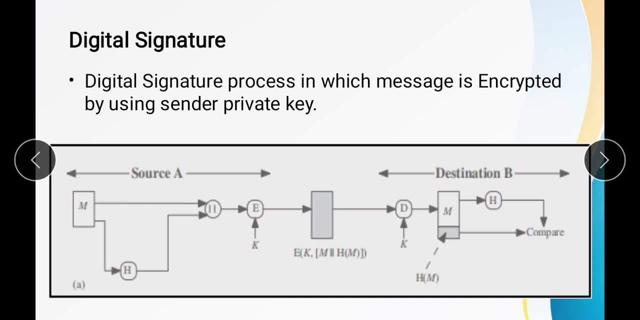 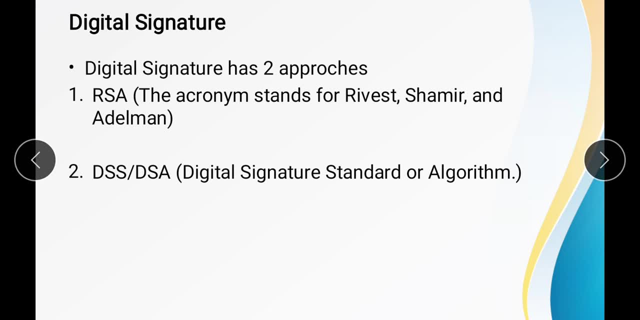 So let us start with the types of the digital signature technique. Digital signature technique can be of two types. So first one is the RSA And second one is the DSA or DSS. So RSA is an acronym stands for Rivest, Shamir and Edelman. 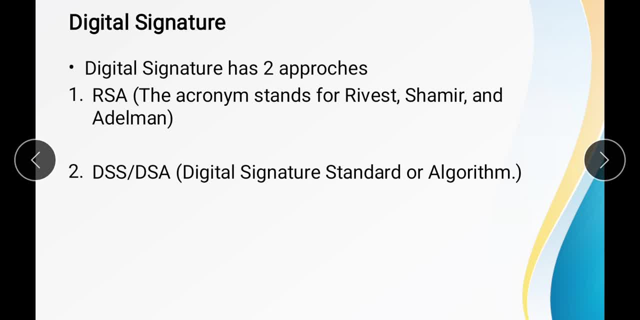 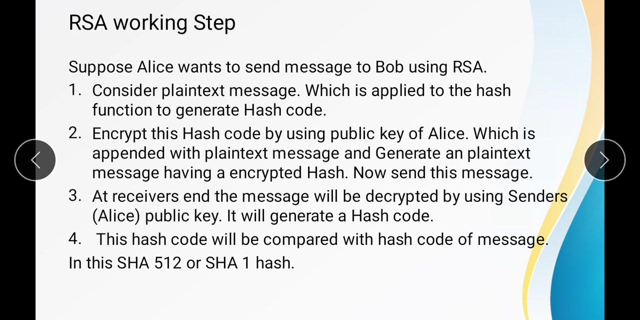 And DSA stands for Digital Signature Standard, Or DSS, that is Digital Signature Standard, And DSA, that is Digital Signature Algorithm. So these are the two types of the digital signature. So let us start with the first one, That is, RSA. 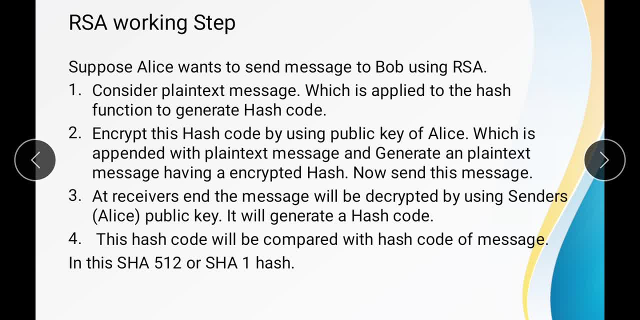 So the working steps of the RSA are given here First. suppose Alice wants to send the message to the Bob using the RSA, So in that case he will follow the following steps for the encryption And decryption as well. So consider the plain text message which is applied to the hash function. 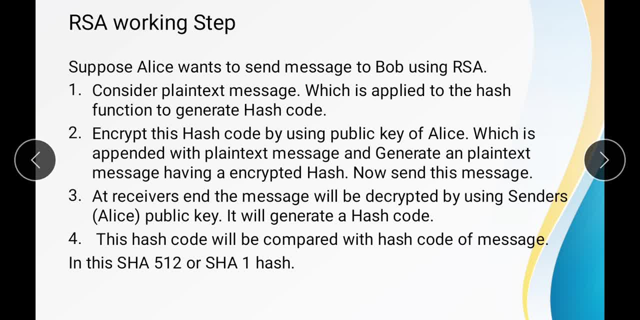 To generate a hash code Here. what we are doing? We are generating a hash code of the message. Now, in second step, that hash code by using the public key- Ok. Hash code is encrypted by using the public key- Ok. And public key of the Alice. 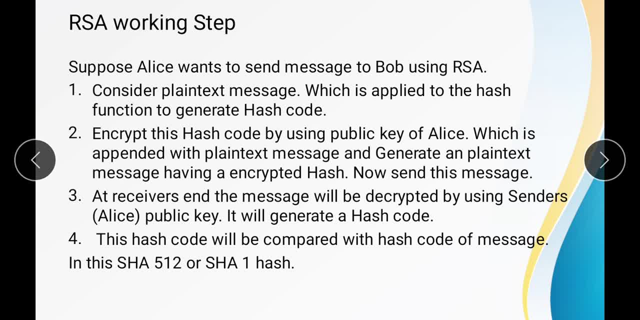 Which is append to the plain text message And generates the plain text message. having the encrypted hash, Now send the message to the. Now send this message to the receiver. Ok, At receiver end. Sorry, My mistake Here not public key. 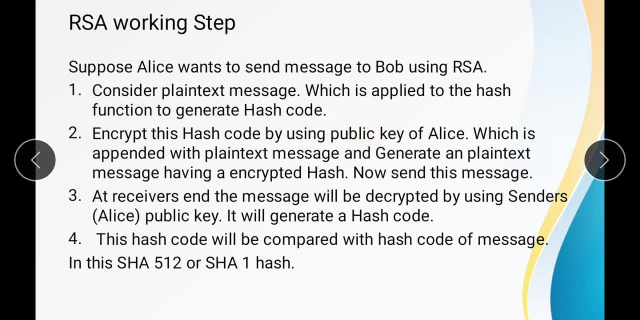 To encrypt the message, we will use the private key. It is a small mistake, So I am correcting it. The hash will be encrypted using the private key, The private key of the Alice. Now, after sending that message to the receiver, 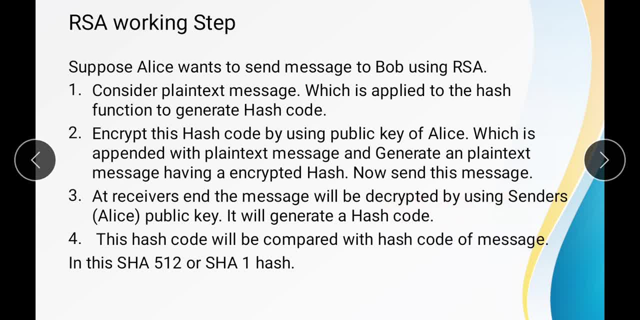 At receiver end. The message will be decrypted by using the senders or Alice public key. So here we are using the public key to the decryption. Here we will use private key for the encryption. Ok Now, after decryption it will generate a hash code. 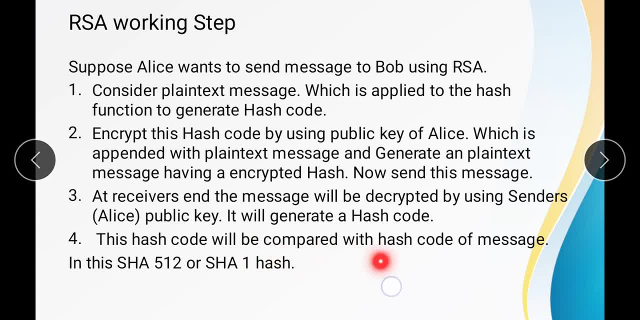 Ok, This hash code will be compared with the hash code of the message. Ok, So if the both hash codes are same, then it is a pure message. Ok, No attacker has attacked the message. Ok, So message is in original form. 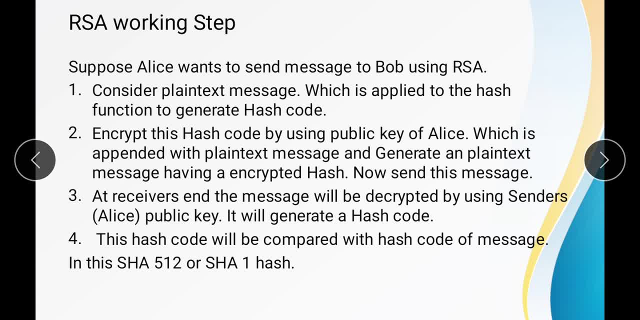 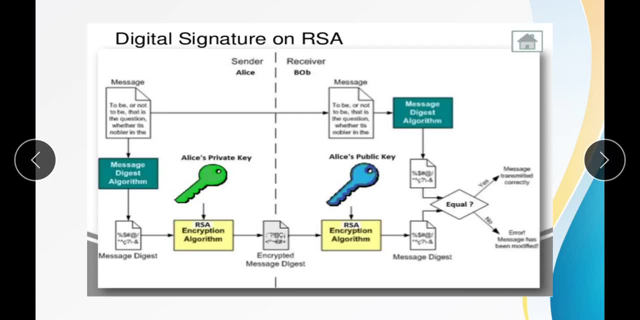 For the hash function. we use sha1 algorithm or sha512 algorithm for the hash function. Ok, So this is the working of the Alice algorithm. You can understand this working using the diagram. So the digital signature on RSE: Ok. 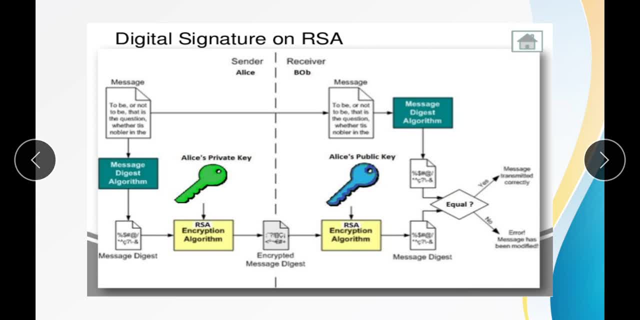 So diagram of the RSE is given here, Ok. So let us start with the Alice that is a sender, and Bob, that is a receiver, Ok, And Alice has a message, Ok. So Alice is doing what he is making a digest. 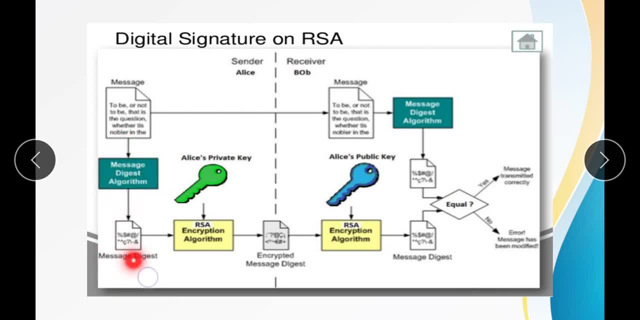 Means he is applying the hash function to generate the hash code. Ok, So that hash code is generated here. Now The hash code is encrypted using the RSE encryption algorithm, or we can say the private key of the Alice. Ok, So Alice private key is used here to encrypt the message. 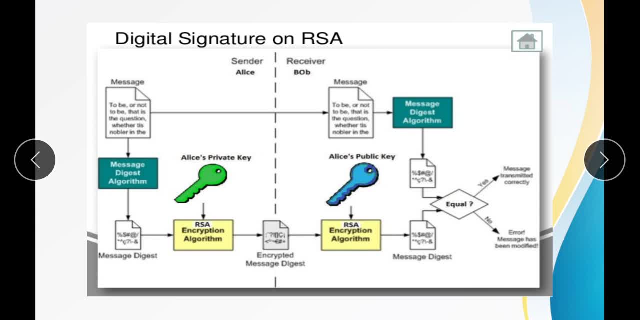 Now this message will be sent to the receiver. Ok, So at the receiver, send message will be decrypted. Or we can say: the decryption is performed here by using the public key of the Alice. So public key of the Alice is used to decrypt the message. 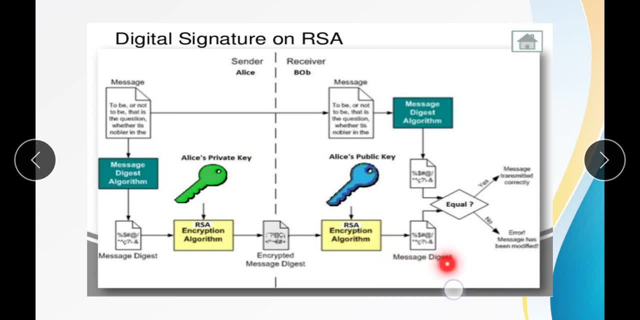 After decrypting the message will get the digest, or that is also known as the hash code. Ok, Now this hash code will be compared with the hash code of the message. Ok, And if the comparison is, the output of the comparison is S. 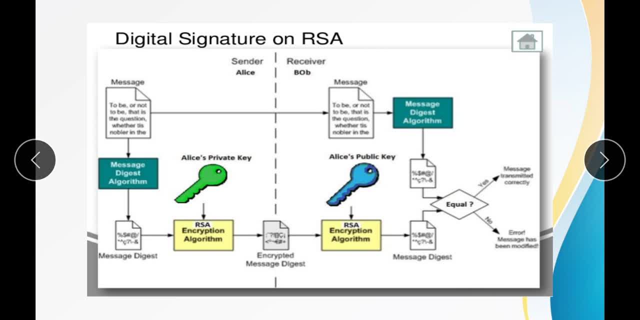 Then it means the message is transmitted correctly Or no means message is not corrupted, Ok. If the answer is no, The output is no. It means that there is error in the message. Message has been modified or forged, Ok. So this is the working diagram of the RSA algorithm. 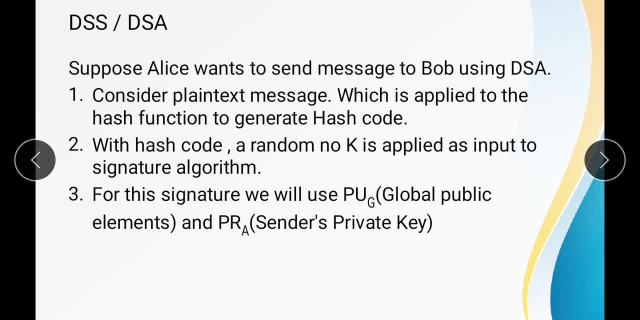 Ok, And as we have mentioned earlier, We use SHA-1 or SHA-512 algorithm For the as a hash function Here. Ok, Now let's start with the second part, that is, DSS or DSC. Ok, So the DSS is the second type of the digital signature. 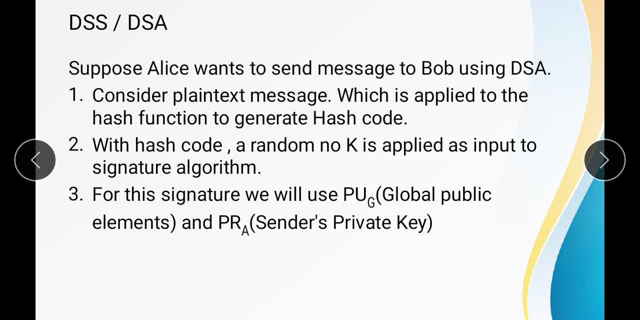 And it is named as digital signature standard Or the digital signature algorithm. Ok, Suppose we have two users, Alice and Bob. Again, Alice wants to send the message to the Bob using DSA. In that case, Consider the plaintext message which is applied to the hash function. 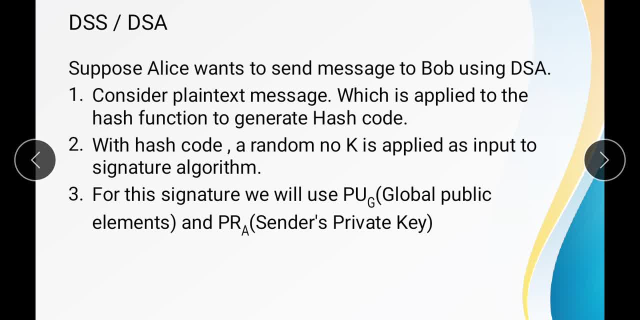 And generated the hash code. Again, what we are doing: We are using the hash function to generate the hash code In the first step. Now, With the hash code, A random number, K is applied. Ok, As a input. And to the signature algorithm. 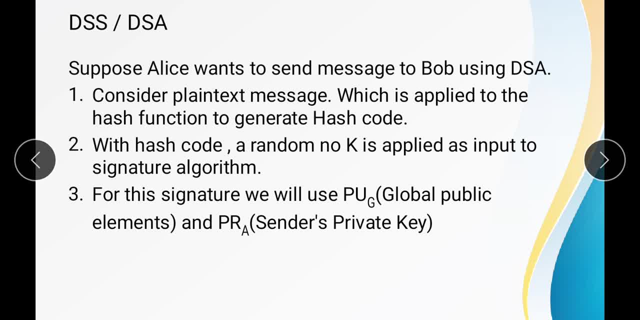 Ok, So what we are doing? We are using a random number, K, And, with hash code, We are applying this number as a input to the signature algorithm. After this, The signature will be used as PUG, That is, global public element. 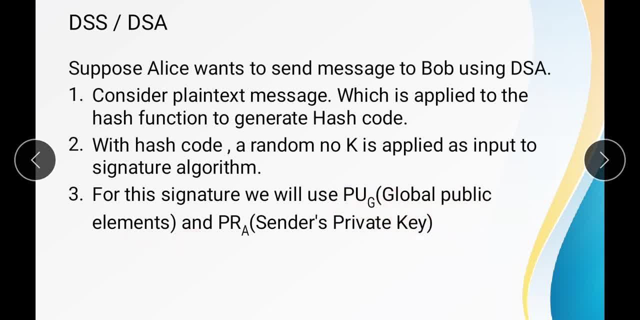 Ok, Global public element, And that can be considered as public key. And second one is PRA, That is sender's private key. Ok, So this is PRA, This is sender's private key And this is public- Global public element. 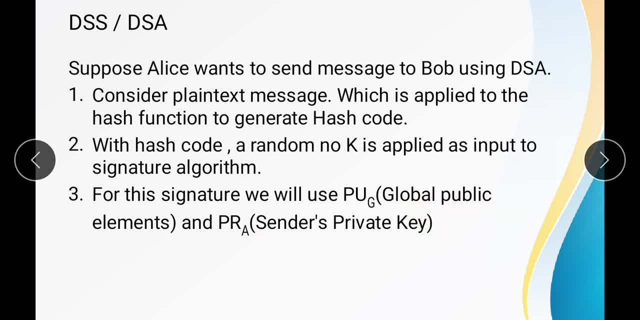 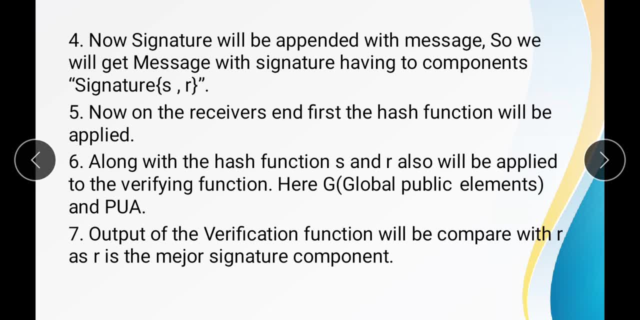 That can be considered as public key. Ok, So these two things we will use for the signature. Next step is Now. signature will be appended with the message Ok. Now Means We generated signature Using hash code and random number. 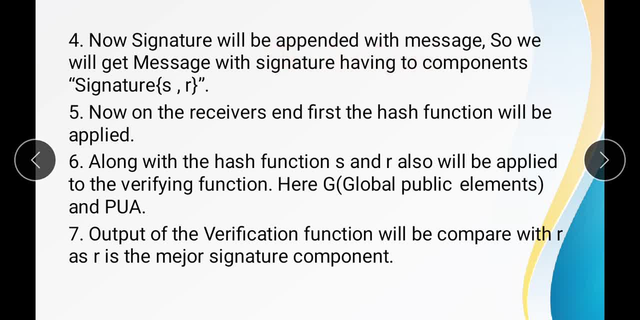 Now That signature will be appended to the message Here, So that will get a message: This is signed. Or we can say that with the signature having the components of S and R Ok. Signature: components S and R Ok. 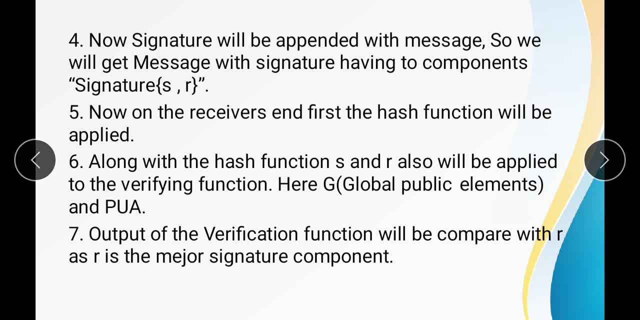 So this is the message. Now We will send this message to the receiver And at the receiver end What will happen. Let's see Now. In fifth step, Now On the receiver's end, First the hash function will be applied. 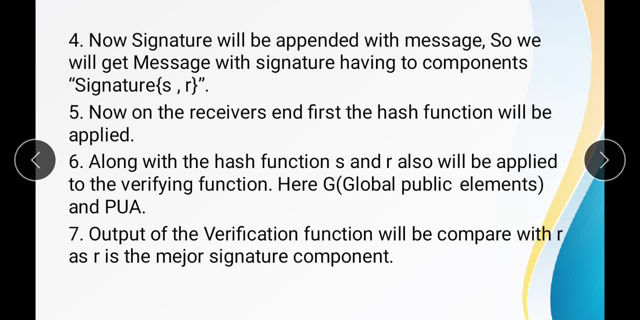 Ok, Six step is Along with the hash function. S and R also will be applied to the To verify the function. Ok, And Here G is the global public element And PUA Will be applied, Ok. 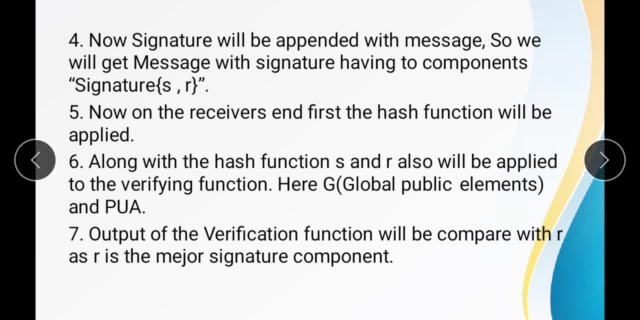 Here We will use these two Means. We will use the public key, of the Public key To Decrypt the function. Ok Output. Ok Now. Now We will send this message to the receiver. Ok, Now. 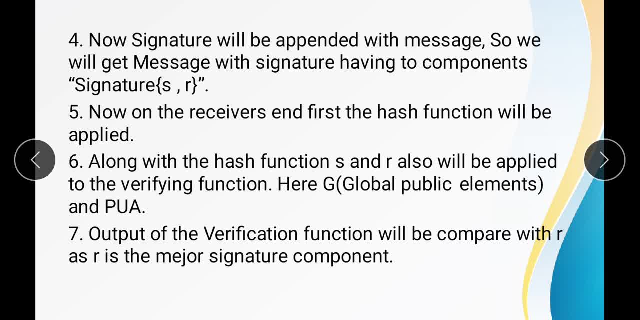 We will send this message to the receiver. Ok, Output of the verification function Will be compared with the R And, As R is The major signature Signature component, Ok, So What we will do After Getting the output of this. 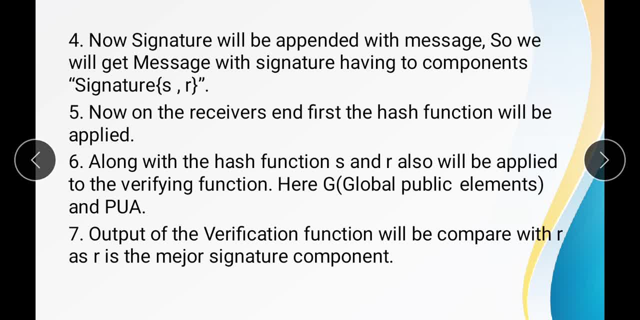 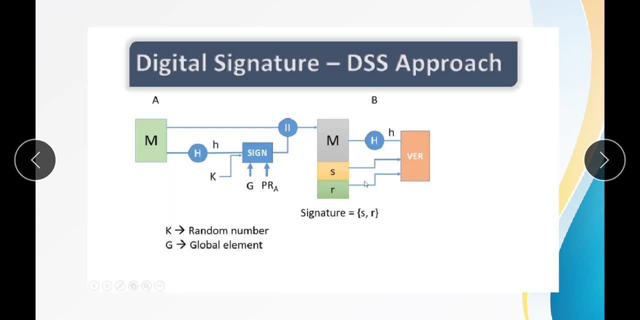 Function Hash function Will Apply. the function Apply the. We will Compare this. That output Means R With the Existing R. So That is, R is the major signature component. Ok, Now We will. 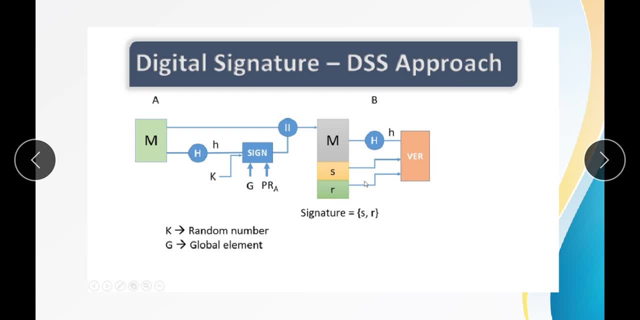 Use the code process Using the Diagram. So What we are doing In the digital signature DSS Approach: Ok, Sender sending the message Using the DSS. So Sender is doing what? First, He applying a. 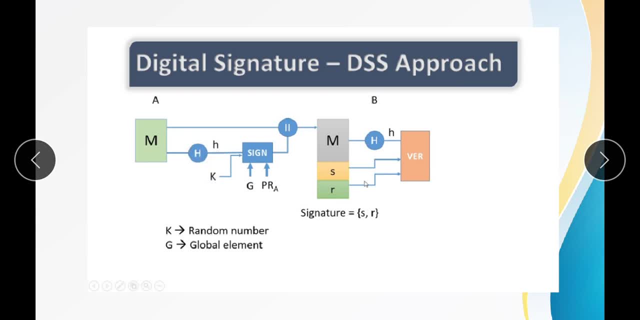 What A Hash Function. To generate a hash code. Ok, Now That hash code Will Will be Combined with The secret key Of the Sender, And for For that We will Use PRA. 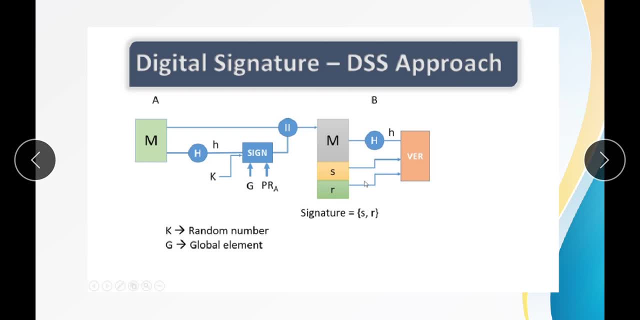 That is The Private Key Or Secret key Of the Sender. Ok, So What we are doing? We are using Three Components, That is, We are sending That. Three Components, That is. 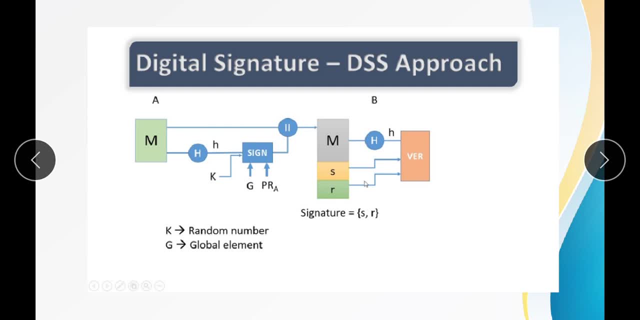 Hash code Sender. Now This Sign, Or Signature, Will be Append To the Message And this Will Come Create A Message That is Looks Like This Message: M. 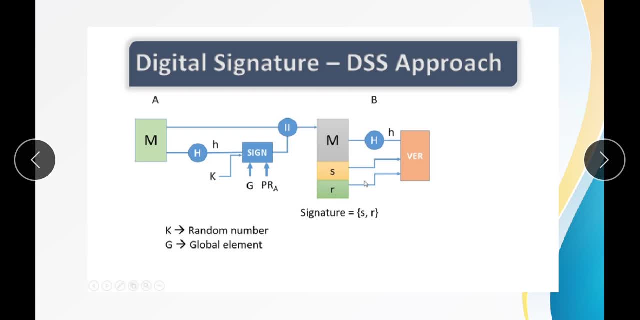 That After That Signature, S And R Will Be S Of The Message And Again R Of The Message, With The R After The Hash And. 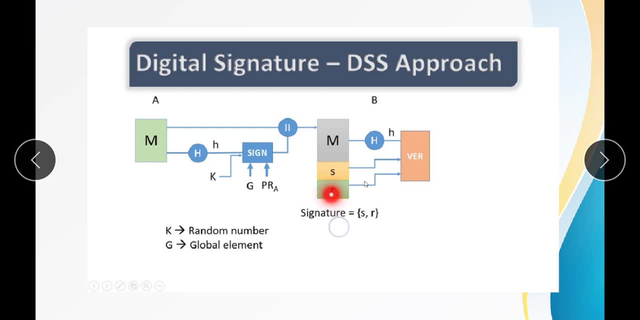 Again R Of The Message, With The R After The Message, Append To The Message. And Again, This Is The Message, The Message Of Message. So 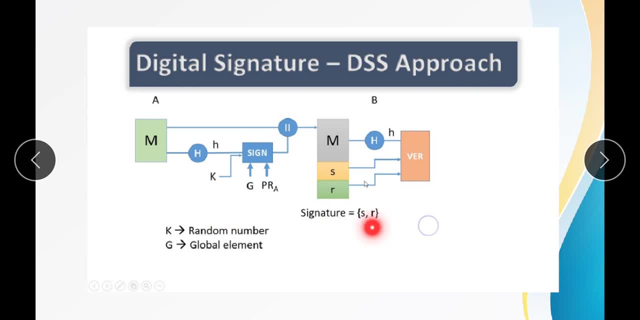 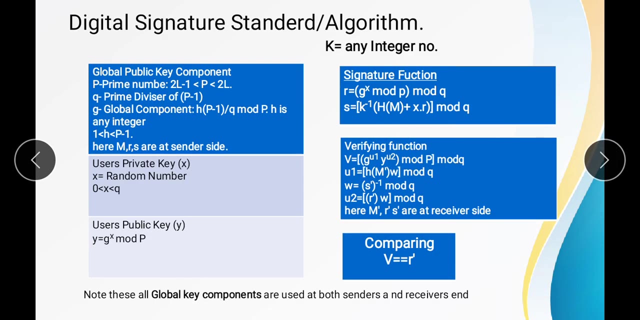 You Can Depend On This Message. After The Message Is The Message Upon RSA and DSA. okay, now let us see the digital signature standard algorithm. okay, so how the algorithm works. so first the global function, key components. okay for. 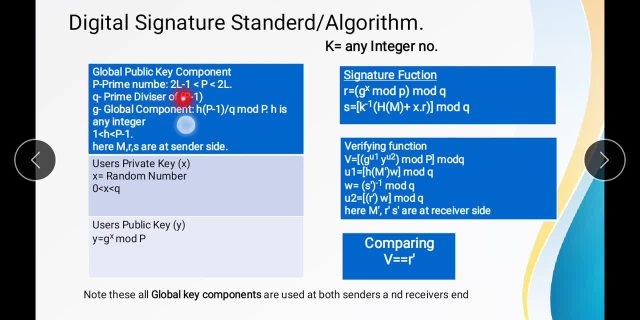 that we use a prime number, that is P. that will be 2 L minus 1, less than P, less than 2 L. okay, so that is the range of the P time number. second, P Q is the prime divisor of the P minus 1. that is a prime divisor, okay. after that, G is the. 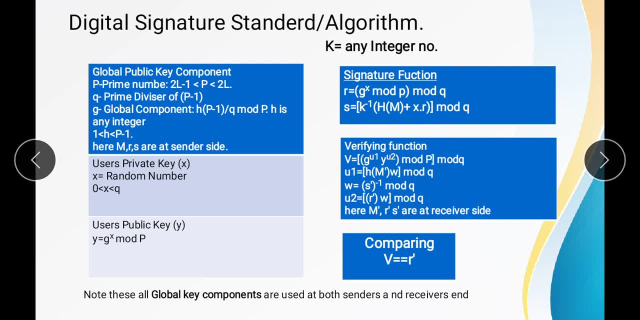 global component, that is equals to H P minus 1 divided by Q mod of P, P into H. okay is the. is any integer okay. okay is any integer. okay is any integer. okay, okay is any integer. okay. this G is any integer that is generated by using this. 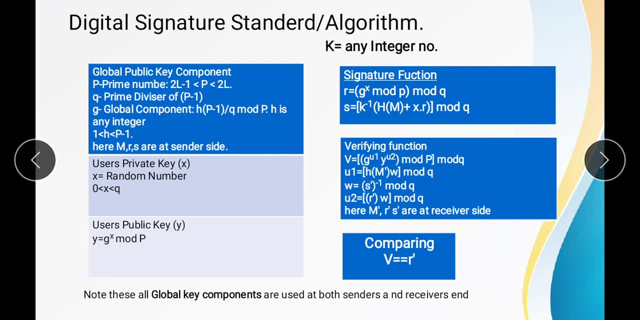 this G is any integer that is generated by using this formula okay. and here again, H has the formula okay. and here again, H has the formula okay. and here again, H has the range H is what? 1 less than H less than P. range H is what? 1 less than H less than P. 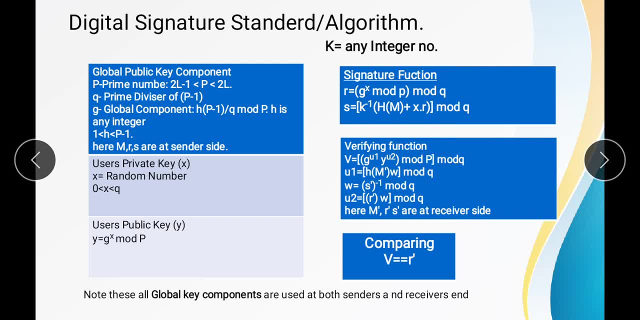 range H is what? 1 less than H, less than P? minus 1, here M are, and yes at the minus 1. here M are, and yes at the minus 1. here M are, and yes, at the sender side. okay, so what are these M is? 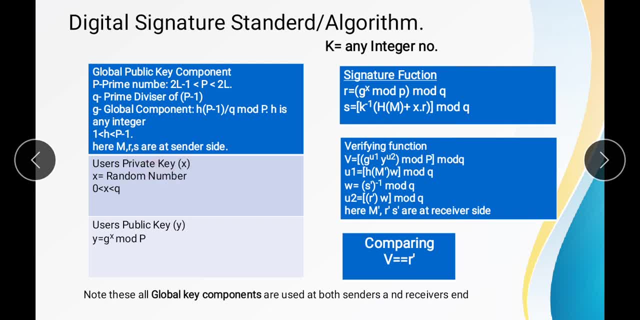 sender side. okay, so what are these? M is sender side okay, so what are these? M is the message: R and S are the major. the message R and S are the major, the message R and S are the major components of the signature. that three components of the signature, that three. 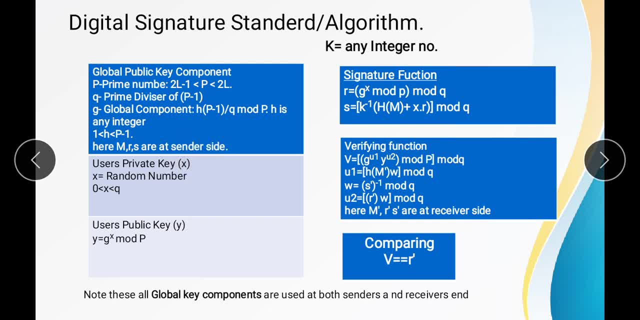 components of the signature. that three things after this whole process will be things after this whole process will be things after this whole process will be sent to the receiver. okay, now use a sent to the receiver. okay, now use a sent to the receiver. okay, now use a private key. how to means what is user. 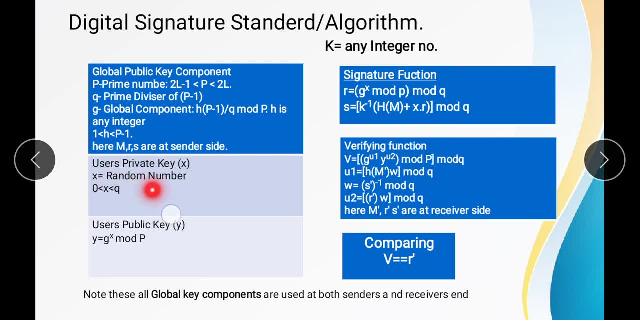 private key. how to means what is user private key? how to means what is user private key? here we use a X- X is a private key. here we use a X- X is a private key. here we use a X- X is a random number, or we have used K actually. 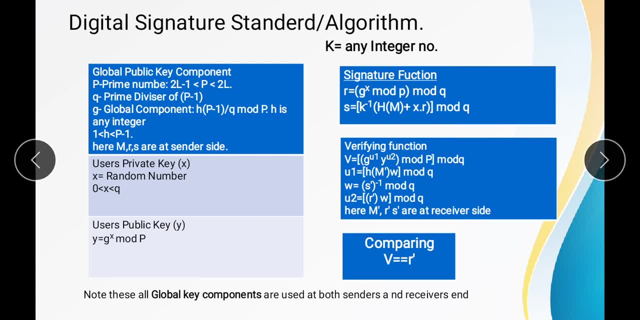 random number, or we have used K actually random number, or we have used K actually in our previous steps. okay, X is a random in our previous steps. okay, X is a random in our previous steps. okay, X is a random number here. X less than 0 and greater. 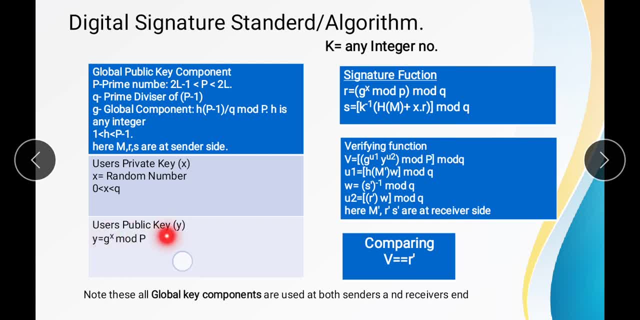 number here: X less than 0 and greater number here X less than 0 and greater than Q. okay, after that. user public key than Q. okay, after that, user public key than Q. okay, after that user public key: again Y, Y will be generated using the. again Y, Y will be generated using the. 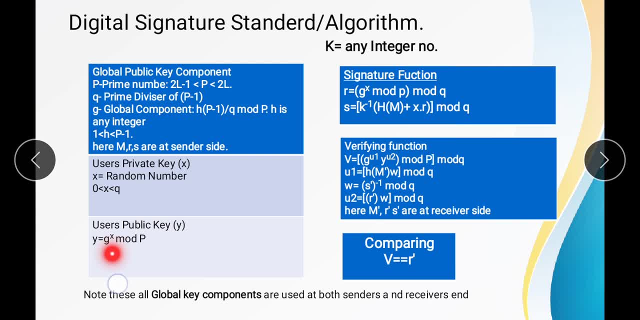 again Y. Y will be generated using the public private king. so Y is equals to G- public private king. so Y is equals to G public private king. so Y is equals to G. rest of our X mod P. okay, next is. rest of our X mod P. okay, next is. 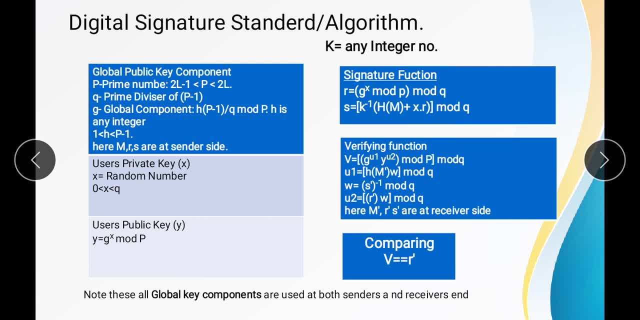 rest of our X mod P. okay, next is signature. function R equals to G rest of signature. function R equals to G rest of signature. function R equals to G rest of our X mod P, mod Q and second signature: our X mod P, mod Q and second signature. 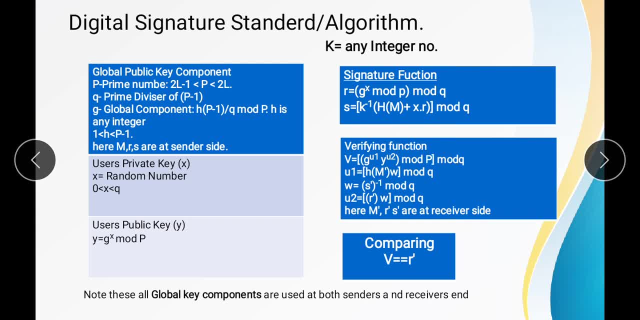 our X mod, P, mod Q and second signature function component that is s. s is function component. that is s: s is function component. that is s s is close to k raise to power minus 1 into hash. close to k raise to power minus 1 into hash. 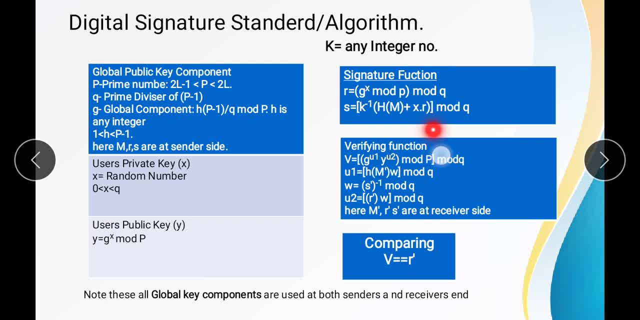 close to k. raise to power minus 1 into hash of M of M of M plus X R mod of Q. okay, so these are the plus X R mod of Q. okay, so these are the plus X R mod of Q. okay, so these are the formulas for the what our signature. 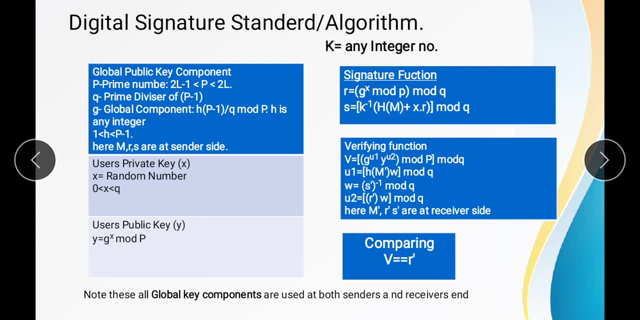 formulas for the what, our signature formulas for the what, our signature function now after signature function. we function now after signature function. we function now after signature function. we have the verify verification function, have the verify verification function, have the verify verification function. so for verification function again, we have 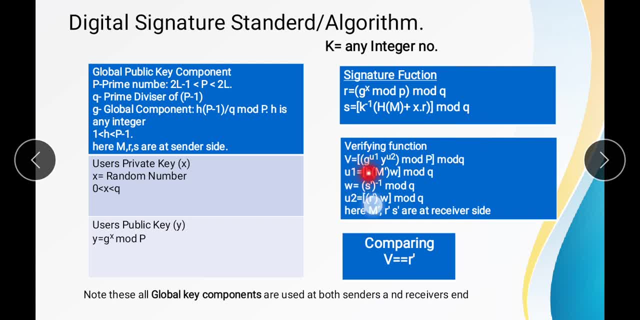 so for verification function again we have. so for verification function, again we have V, that is verification function. where V, that is verification function, where V, that is verification function. where inputs are G raise to power u raise to inputs. are G raise to power u raise to inputs. are G raise to power u raise to power minus 1 into y raise to power u. 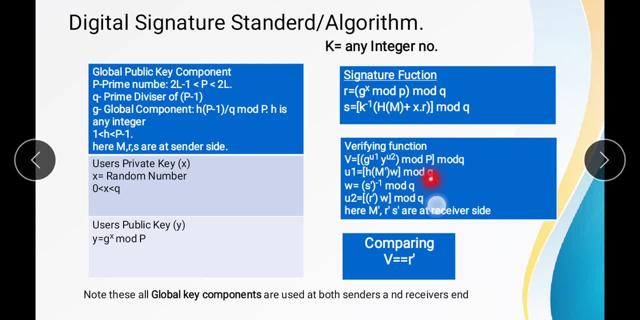 power minus 1 into y- raise to power. u power minus 1 into y- raise to power. u raise to raise to power. u raise to power. u 2 mod P mod Q. so this is the first. 2 mod P mod Q. so this is the first. 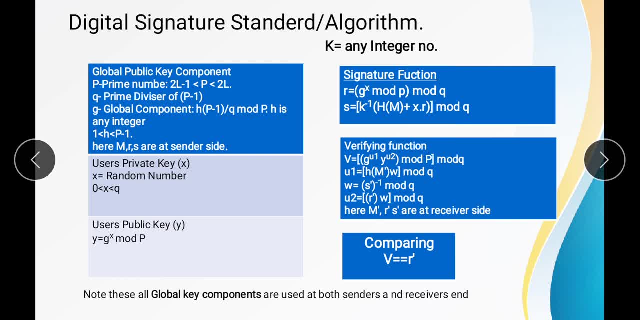 2 mod P, mod Q. so this is the first formula of V. that is verification formula of V. that is verification formula of V. that is verification function, verifying function. after that u function, verifying function. after that u function, verifying function. after that u: 1. how to calculate u 1. so u 1 is equals. 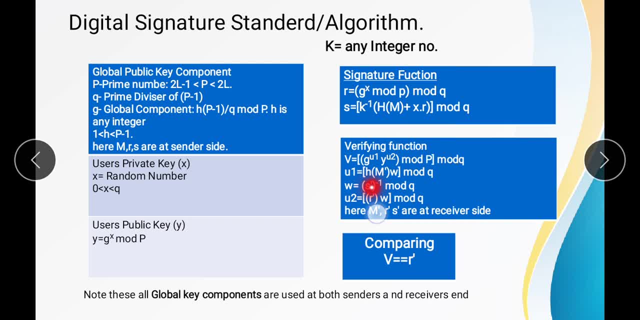 1. how to calculate u 1, so u 1 is equals 1. how to calculate u 1, so u 1 is equals to hash of message. inverse here here M to hash of message. inverse, here here M to hash of message inverse, here here M is M inverse actually here we have use M. 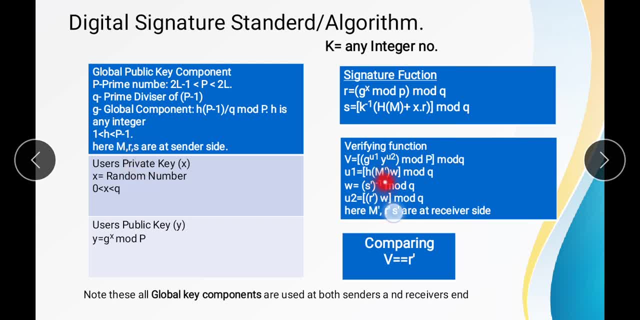 is M inverse? actually here we have use M. is M inverse? actually here we have use M and this is M inverse. okay, so H of M and this is M inverse. okay, so H of M and this is M inverse. okay, so H of M inverse W mod Q. now we have to calculate. 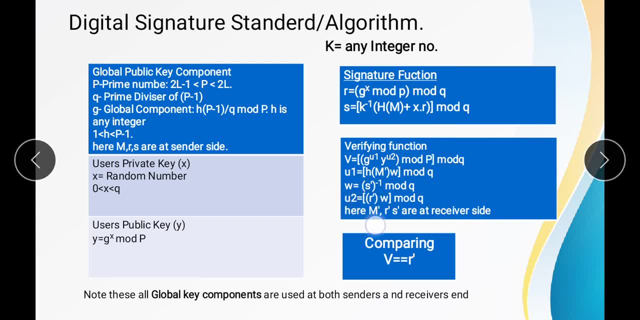 inverse W mod Q. now we have to calculate inverse W mod Q. now we have to calculate W, so W equals to s inverse. again we have W, so W equals to s inverse. again we have W, so W equals to s inverse. again we have used here s, but this is s inverse. so this: 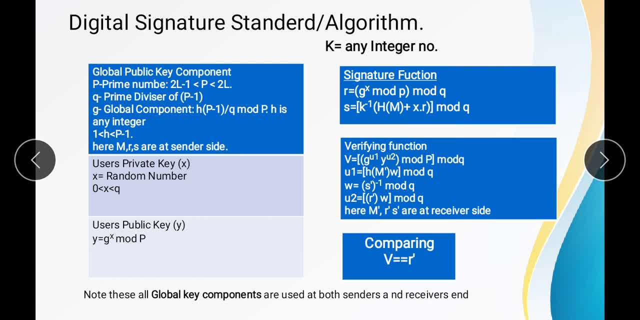 used here s, but this is s inverse. so this used here s, but this is s inverse. so this is that receiver send this was a at. is that receiver send this was a at. is that receiver send this was a at sender send so s inverse. sorry s dash. 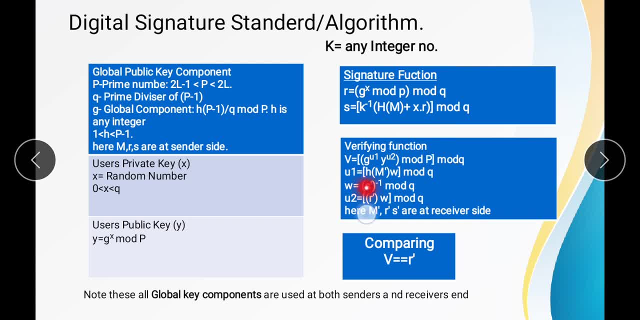 sender. send so s inverse sorry s dash. sender. send so s inverse sorry s dash. inverse mod M: okay, so this is it okay. inverse mod M: okay, so this is it okay. inverse mod M okay, so this is it okay. after that, you, you two, we have to. 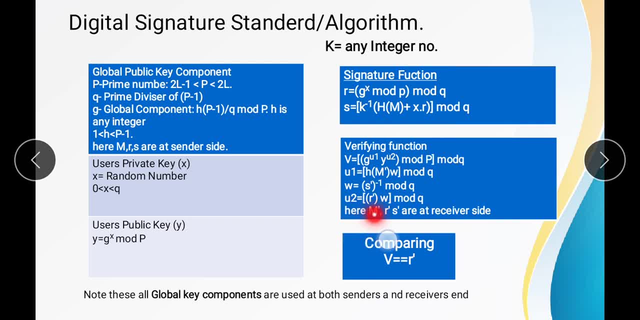 after that, you, you two, we have to. after that, you, you two, we have to calculate you two as well. so you two calculate you two as well. so you two calculate you two as well. so you two goes to R dash into W mod Q. so here we. 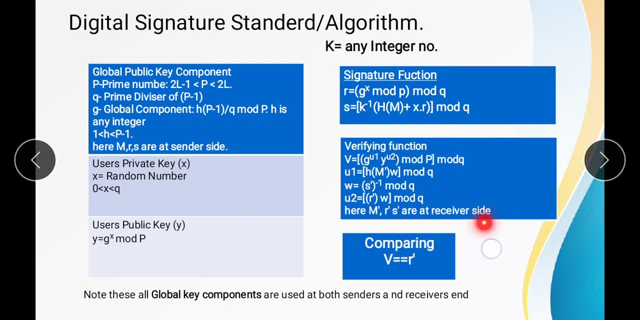 goes to R dash into W mod Q. so here we goes to R dash into W mod Q. so here we have M dash, R dash and S dash. these are: have M dash, R dash and S dash. these are: have M dash, R dash and S dash. these are at the receiver end. okay, so we have to. 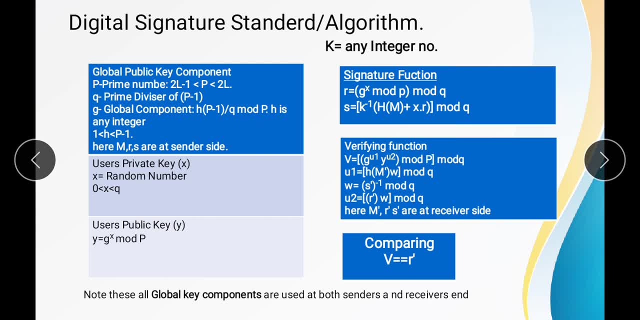 at the receiver end. okay, so we have to at the receiver end. okay, so we have to calculate this at sender and sender send. calculate this at sender and sender send. calculate this at sender and sender send. we have to calculate these all things at. we have to calculate these all things at: 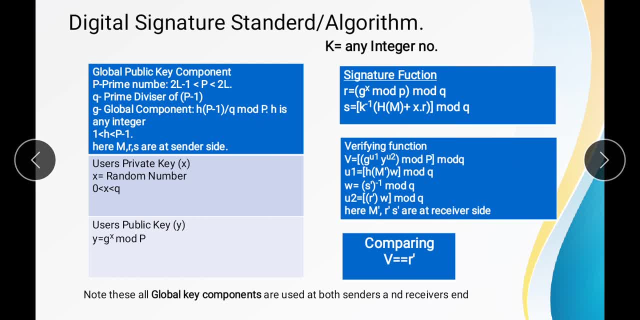 we have to calculate these all things at the receivers and after these things we the receivers, and after these things we the receivers. and after these things we have to compare V equals to equals to R. have to compare V equals to equals to R. have to compare V equals to equals to R means V. that is verification function. 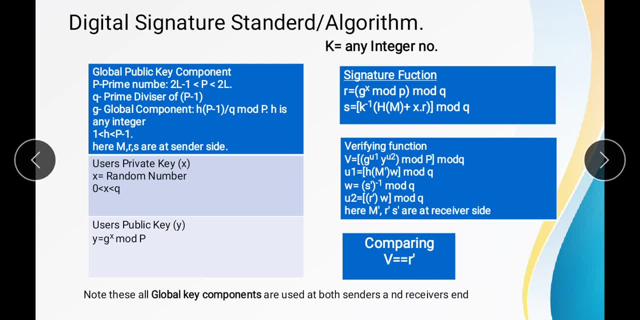 means V, that is verification function. means V, that is verification function. this must be equal, equals to R dash. so this must be equal, equals to R dash. so this must be equal, equals to R dash. so R dash of the receiver must be same with R dash of the receiver must be same with. 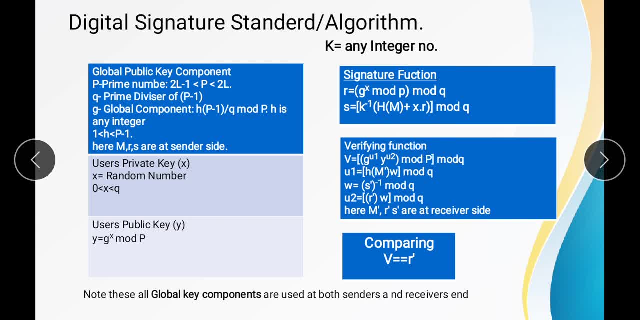 R dash of the receiver must be same with the V. if the comparison is true, then the V. if the comparison is true, then the V. if the comparison is true, then message is not corrupted and in the raw message is not corrupted and in the raw message is not corrupted and in the raw form. if the verification is wrong, then 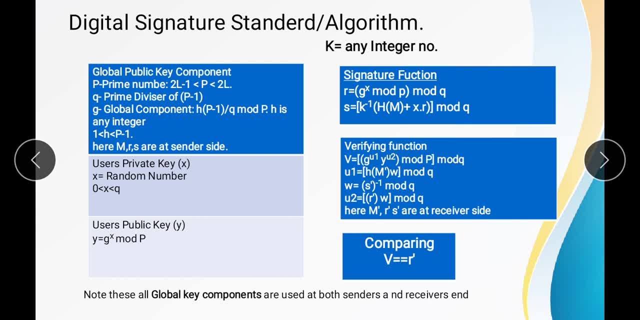 form. if the verification is wrong, then form. if the verification is wrong, then message is corrupted. so this is the whole message is corrupted. so this is the whole message is corrupted. so this is the whole idea of the digital signature standard, idea of the digital signature standard, idea of the digital signature standard algorithm. okay, so these are some review. 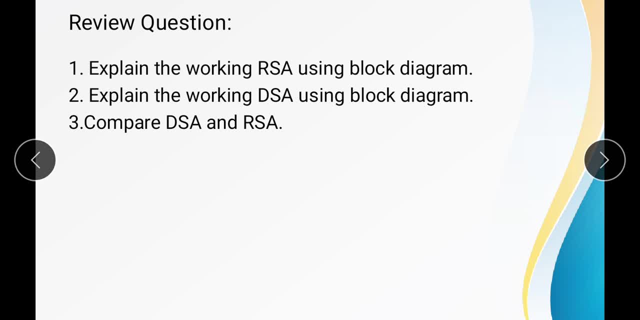 algorithm. okay. so these are some review algorithm. okay. so these are some review questions. okay. so I hope all the questions okay. so I hope all the questions okay, so I hope all the students will be able to give the answers. students will be able to give the answers. 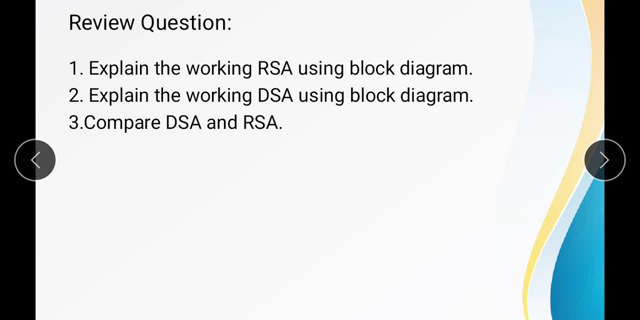 students will be able to give the answers of this review questions after the of this review questions. after the of this review questions after the lecture. after the learn after learning lecture. after the learn after learning lecture. after the learn after learning the lecture properly. okay, so the first. 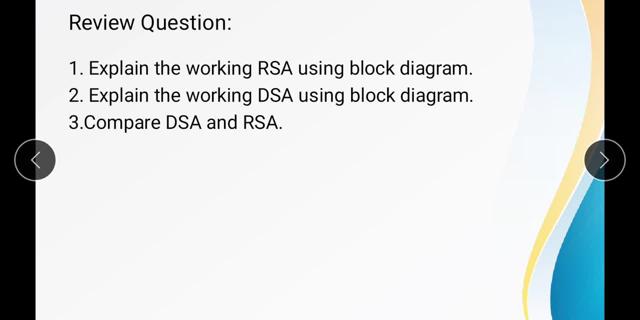 the lecture properly okay. so the first the lecture properly okay. so the first question is: explain the working of RSA. question is: explain the working of RSA. question is: explain the working of RSA with the block diagram or using block with the block diagram or using block with the block diagram or using block diagram. explain the working of DSA using 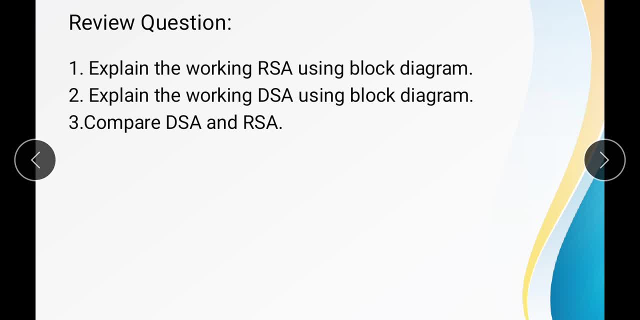 diagram. explain the working of DSA using diagram. explain the working of DSA using the block diagram. and compare DSA and the block diagram. and compare DSA and the block diagram. and compare DSA and RSA. okay, so these were the questions- RSA. okay, so these were the questions. 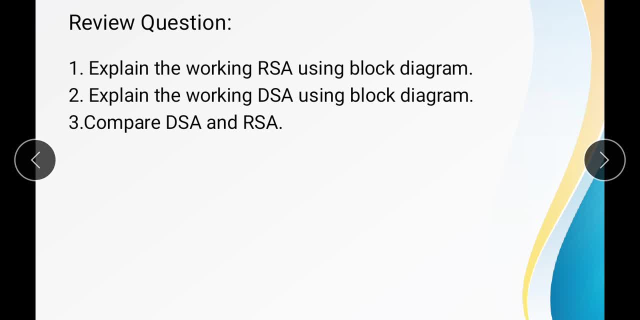 RSA. okay, so these were the questions. okay, I think all will be able to give. okay, I think all will be able to give. okay, I think all will be able to give the answers of this. all questions, again. the answers of this. all questions, again, the answers of this, all questions again. I am repeating that digital signature is. 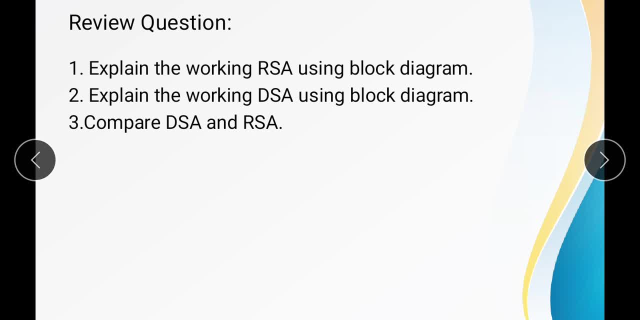 I am repeating that digital signature is. I am repeating that digital signature is what it is a technique. see this one line, what it is a technique. see this one line, what it is a technique. see this one line is very important. it is a technique in is very important. it is a technique in. 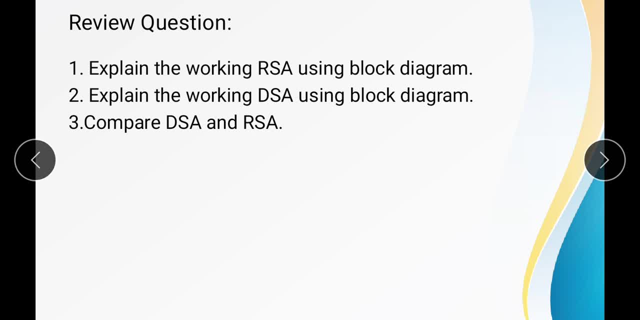 is very important. it is a technique in which sender use its own private key, to which sender use its own private key, to which sender use its own private key to send the message and receiver use the send the message and receiver use the send the message and receiver use the public key to decrypt the message. means 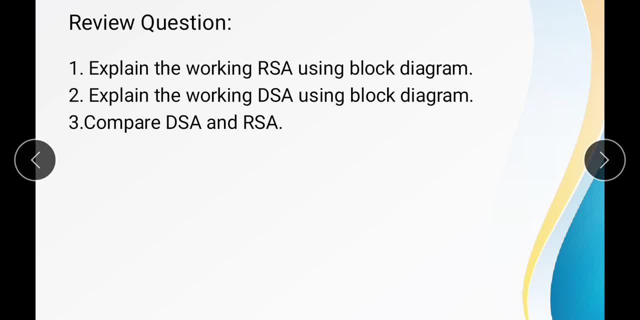 public key to decrypt. the message means public key to decrypt. the message means for encryption: we are using private key for encryption. we are using private key for encryption. we are using private key for decryption. we are using public key for decryption. we are using public key for decryption. we are using public key. okay, thank you so much, guys. I hope you. 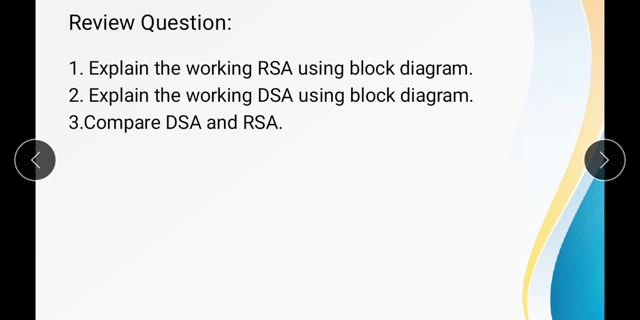 okay, thank you so much, guys. I hope you okay. thank you so much, guys. I hope you will be. you have. you are enjoying the will be you have. you are enjoying the will be. you have. you are enjoying the lectures. thank you so much. 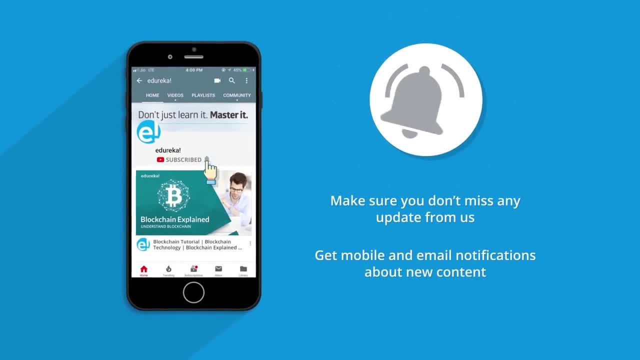 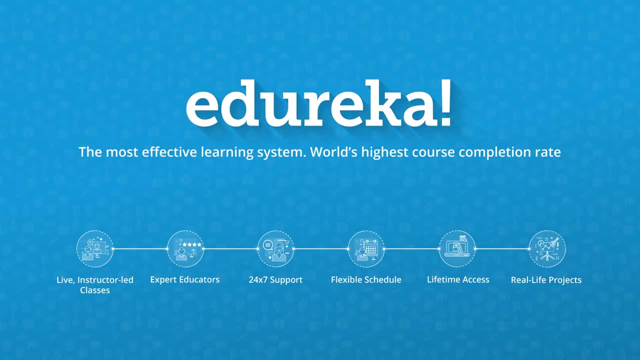 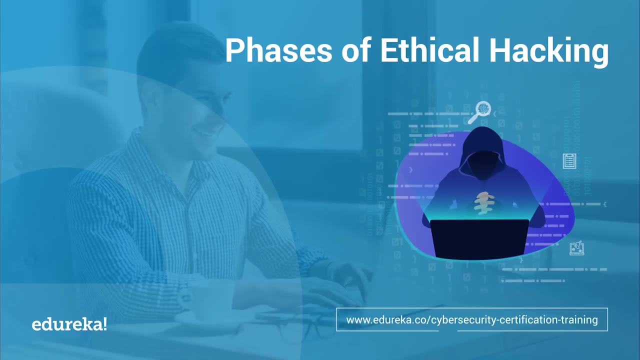 Hi everyone, this is Omkar from Edureka, and today I'll be speaking about different phases of ethical hacking. Well, if you're watching this video, I'm sure you want to learn hacking and become an ethical hacker. But if that's the case, it's a very good thing, because ethical